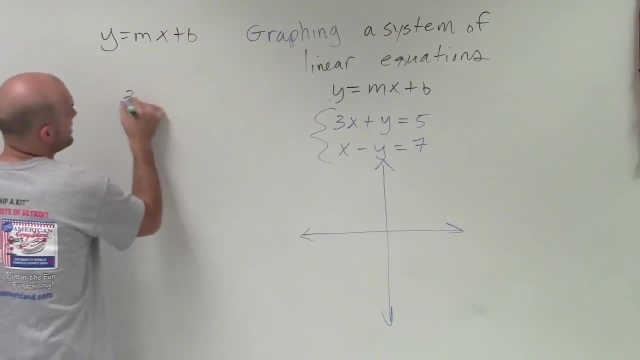 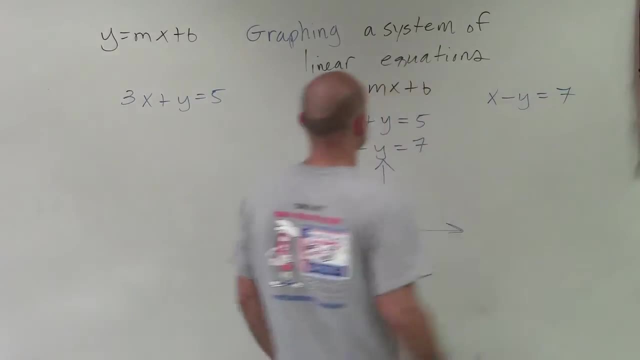 y intercepts method if I'd like to, but I think these are going to be better suited for us to solve by converting them to slope intercept form. So to convert to slope intercept form, which is right here, we need to isolate our variable y. So what I like to do sometimes, 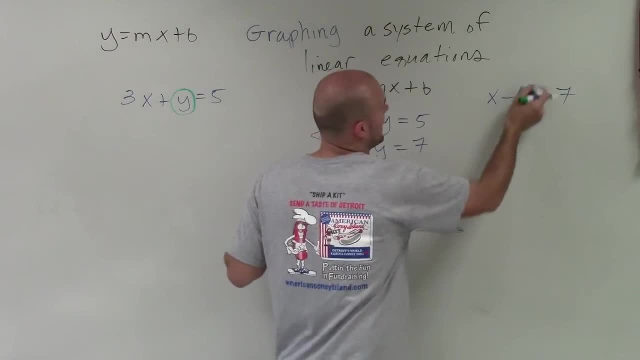 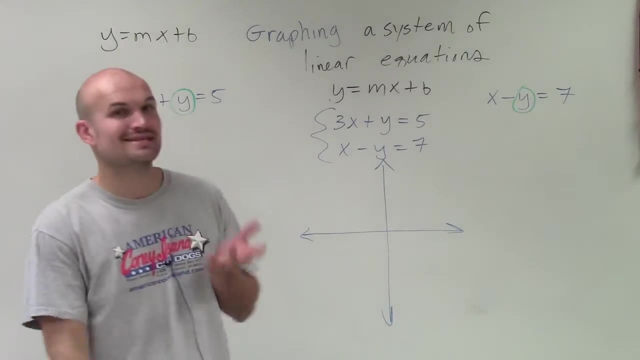 is circle the y. So therefore, that's going to tell me I need to undo everything that's happening to that, just like we solve our literal equations. So the first thing we always undo is addition and subtraction. And I look at this and I notice: all right, we're going. 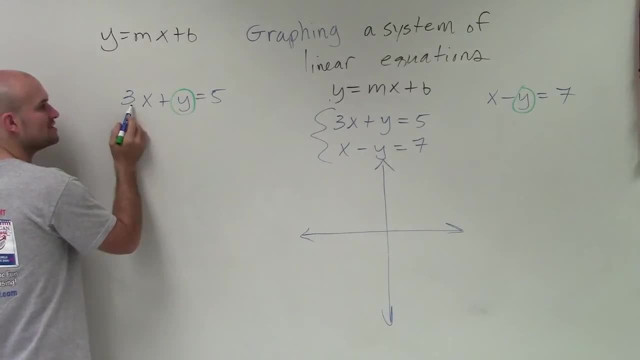 to have a plus sign. Well, I see a plus sign, but what's being added or subtracted to the y? Well, this 3x is. And just to kind of prove my point, if I rewrote this, I could rewrite: 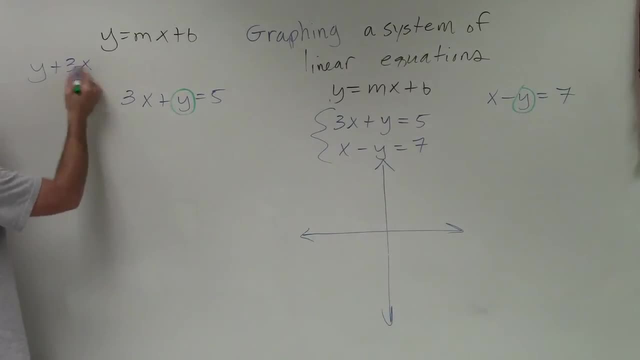 this as y plus 3x, right, Because that 3x is positive, So it's going to be a plus of 3x. Therefore, to undo the addition of 3x, I need to subtract 3x on both sides. Well, 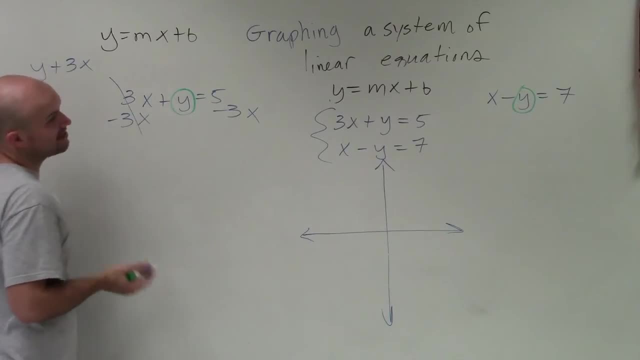 positive 3x minus 3x. that adds up to 0.. 0x, which is just 0.. So therefore, I'm left with a y equals 5 minus 3x. Now, this will be the last time I'm probably going to be able to. 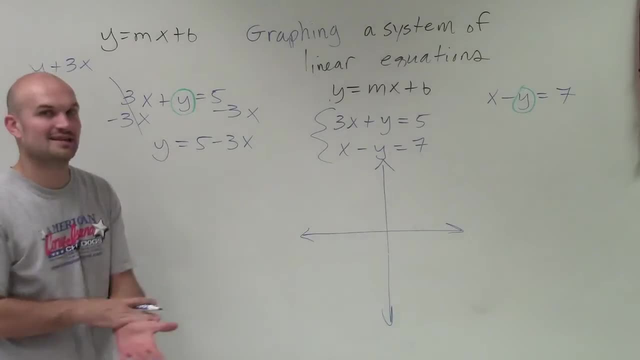 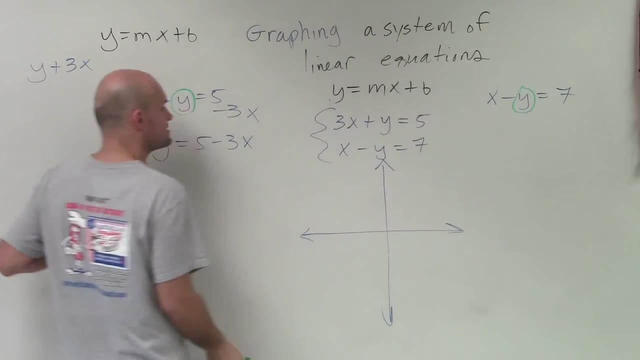 it as 5 minus 3x. However, we want to convert it back to mx plus b form. Therefore, we want the 3x to be in front of the 5. So make sure, though, it's a minus 3x. So when I rewrite. 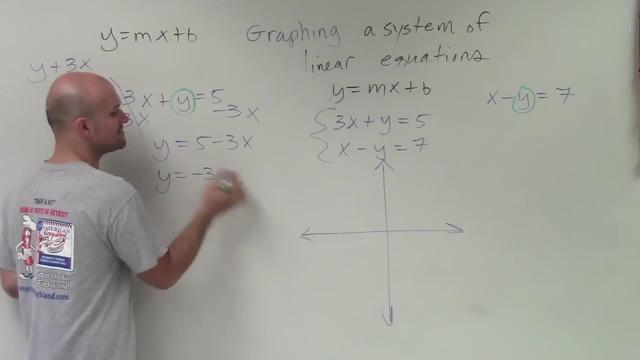 this. I'm going to take that sign with it. And then the 5 is positive, so it would be plus 5.. Now I have an equation where I know my y-intercept is at 0 comma 5, and my slope 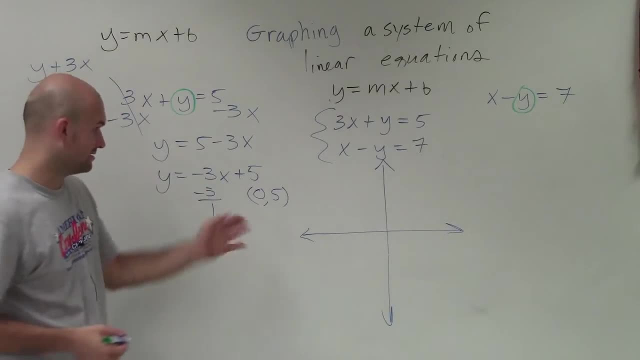 is at negative 5.. So I'm going to do this, I'm going to do this, I'm going to do this. Negative 3 over 1, right, Because, remember, b is your y-intercept, which is a coordinate. 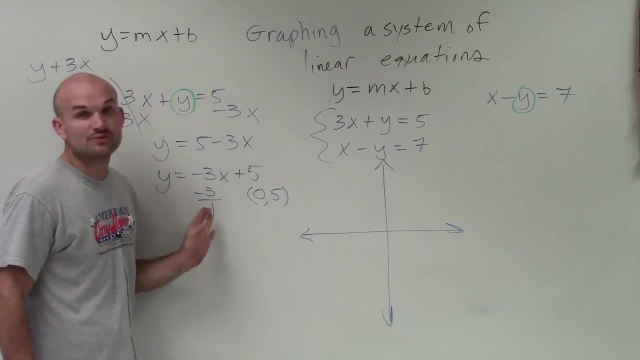 point and slope is your rate of change, which we write as a fraction. So now to graph this, I go up 5.. 1,, 2,, 3,, 4,, 5.. And now, since my rate of change is negative, it can either. 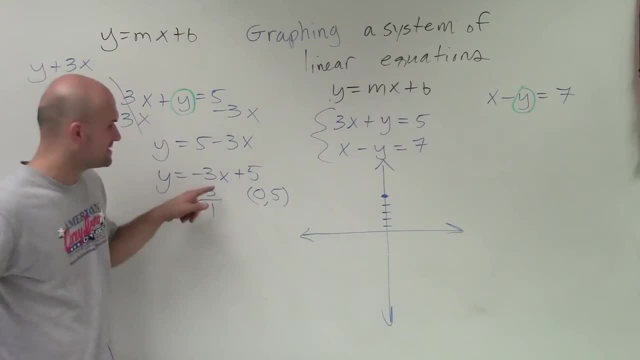 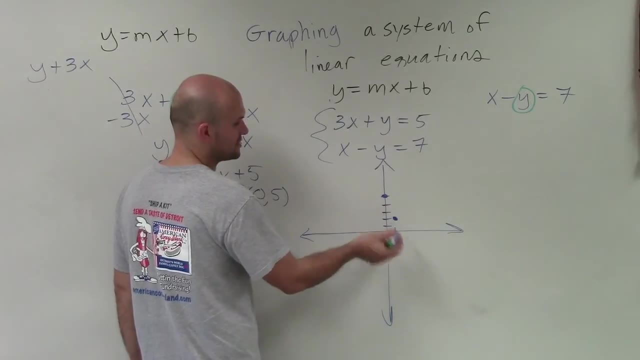 be negative up top or in the bottom, It doesn't really matter. But if I keep the negative sign up top, that's going to tell me to go down 3, and then that's in the negative direction and then over 1 in the positive direction, I could also go up 3 in the positive. 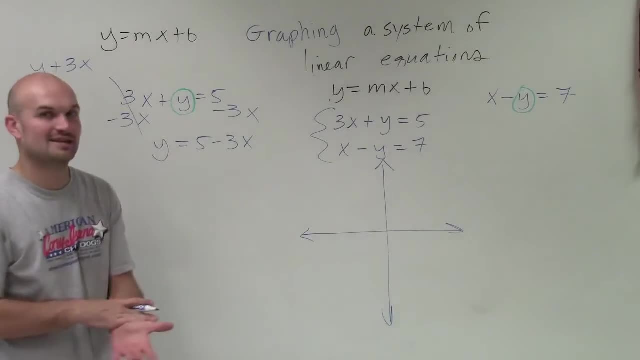 do this, So I'm going to do this, So I'm going to do this, So I'm going to do this. So I'm probably going to do this without immediately making the correction. However, I want you to see it, because a lot of students want to write it as 5 minus 3x. However, we want to 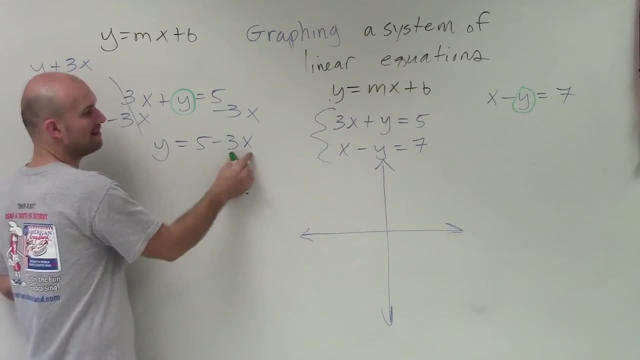 convert it back to mx plus b form. Therefore, we want the 3x to be in front of the 5.. So make sure, though, it's a minus 3x, So when I rewrite this, I'm going to take that sign. 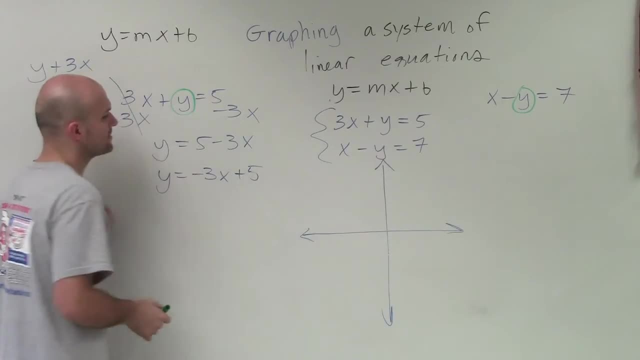 with it, And then the 5 is positive, so it would be plus 5.. Now I have an equation where I know my y-intercept is at 0 comma 5, and my slope is at negative 3 over 1. Because, remember, b is your y-intercept, which is a coordinate point, And slope is 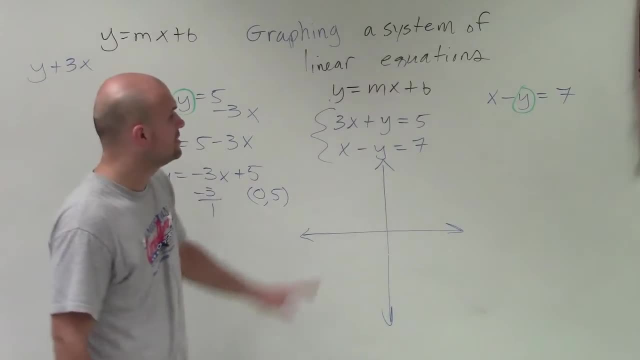 your rate of change, which we write as a fraction. So now to graph this, I go up 5.. 1,, 2,, 3,, 4,, 5.. And now, since my rate of change is negative, it can either be negative up top: 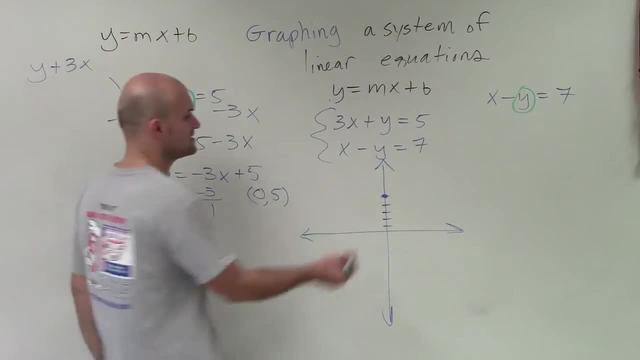 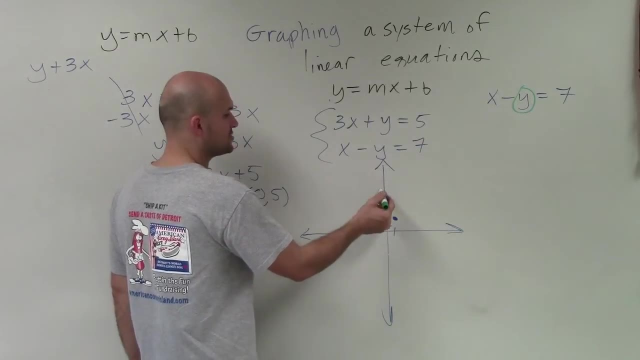 or in the bottom, It doesn't really matter. But if I keep the negative sign up top, that's going to tell me to go down 3. And then that's in the negative direction And then over 1 in the positive direction. I could also go up 3 in the positive direction. I could also. 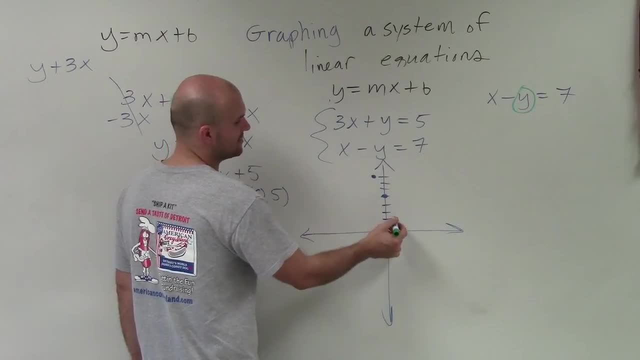 go up 3 in the positive direction but then left 1 in the negative to still keep my slope negative. All right, So there's just a rough sketch of that first equation. Now I need to graph this equation, So I need to isolate it Again. I have the addition of the x, So I'm going. 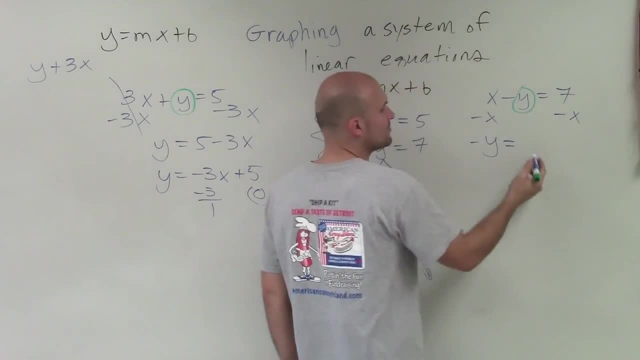 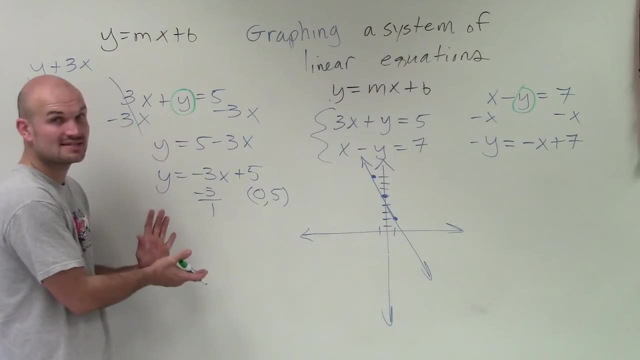 to subtract the x, Then I have negative y equals. Now I'm just going to rewrite it how it should be without having to go through all those extra steps and explanations, Because hopefully you can see why I wrote the negative x in front of the positive 7. But now I have 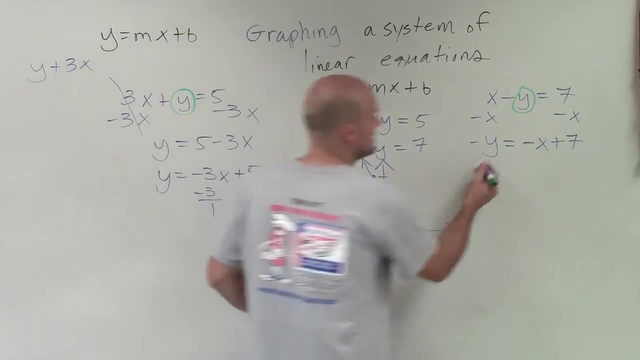 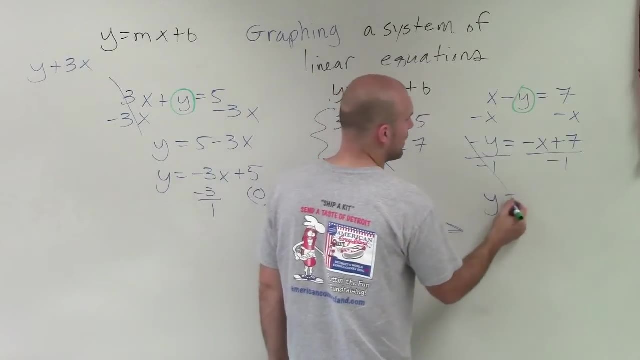 this negative y. I need to solve for y, not negative y. So I'll divide by negative 1.. Now it's really important when we do this: negative divided by negative, those will divide into 1.. So I'm left with y equals. Be careful When I'm dividing this. I need to make sure I divide. 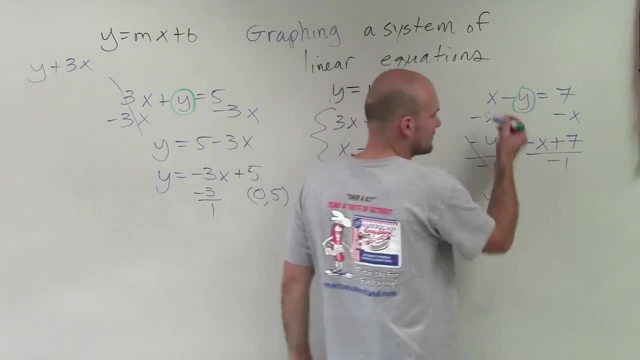 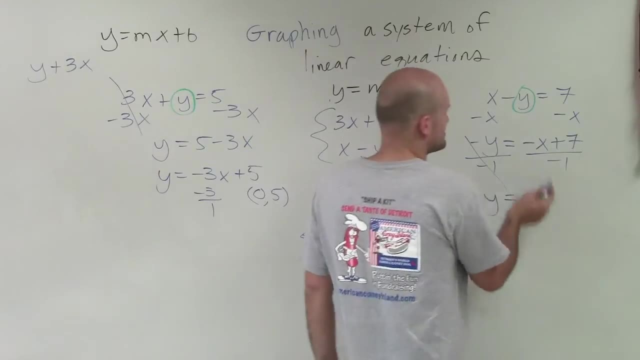 the negative 1 into both of my terms. Since they're separated by addition, or if they're separated by subtraction, you have to make sure you divide into both of the terms. So therefore now I'll have a positive x minus 7.. 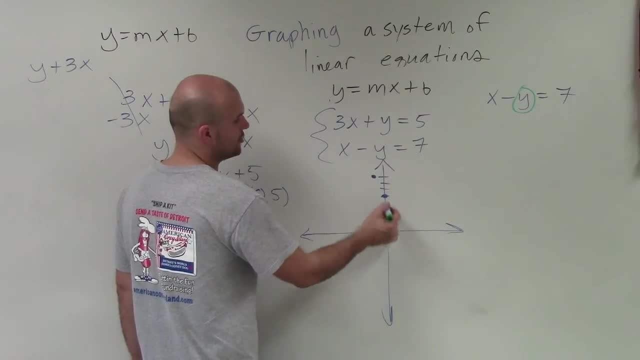 direction but then left 1 in the negative to still keep my slope negative. All right, So there's just a rough sketch of that first equation. Now I need to graph this equation, so I need to isolate it Again. I have the addition of the x, so I'm going to subtract. 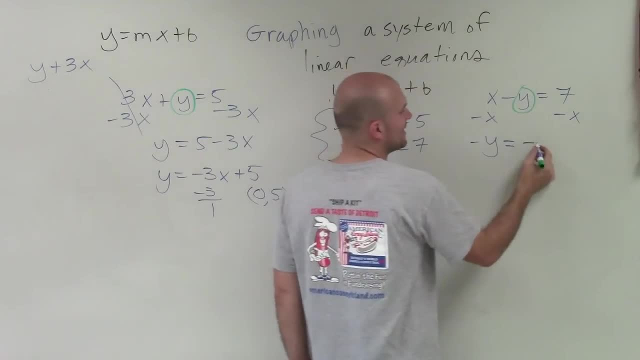 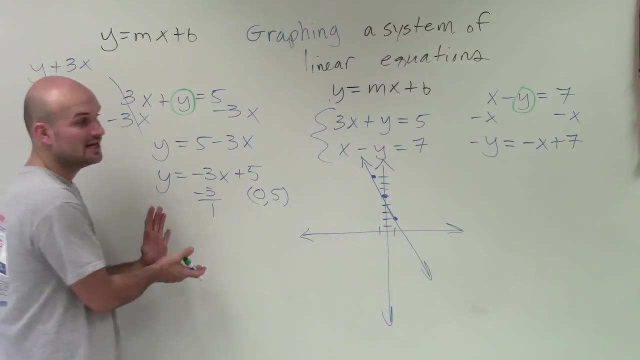 the x, Then I have negative y equals. Now I'm just going to rewrite it how it should be all right, without having to go through all those extra steps and explanations, because hopefully you can see why I wrote the negative x in front of the positive 7. But now I have 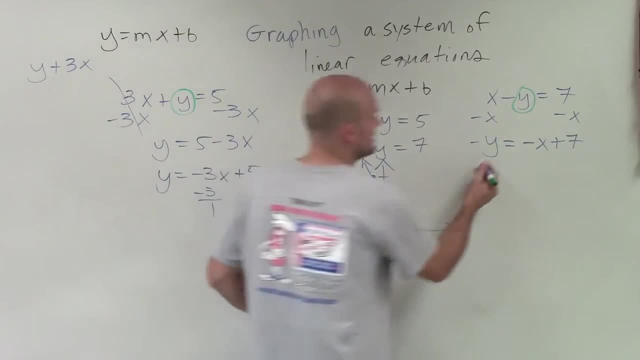 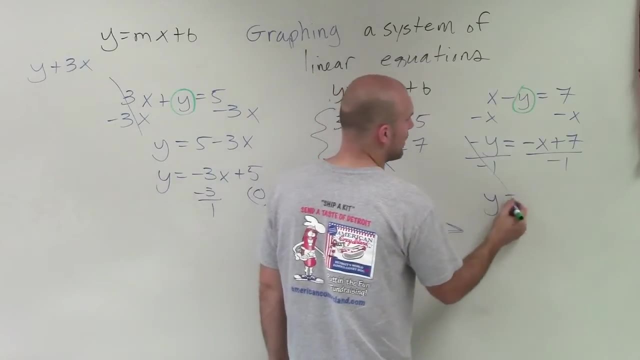 this negative y. I need to solve for y, not negative y, So I'll divide by negative 1.. Now it's really important when we do this: negative divided by negative, those will divide into one. So I'm left with y equals. Be careful when I'm dividing this. I need to make sure. 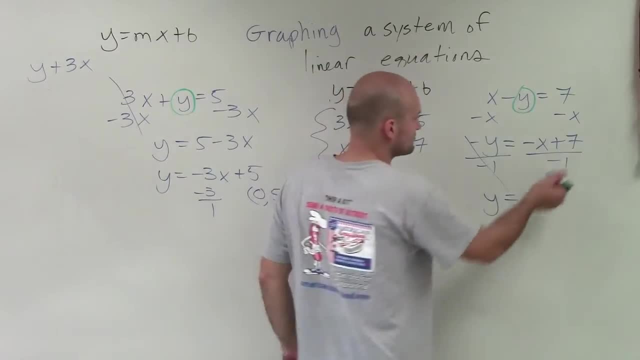 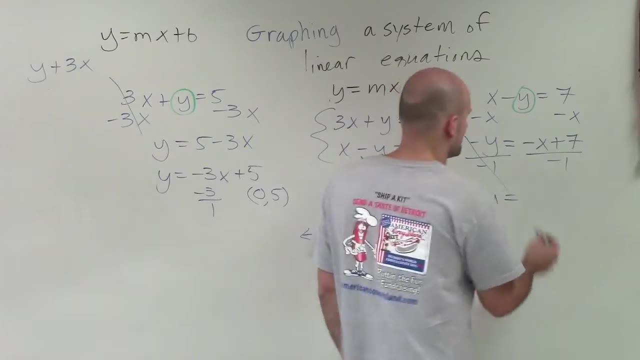 I divide the negative 1 into both of my terms. Since they're separated by addition, or if they're separated by subtraction, you have to make sure you divide into both of the terms. So therefore, now I have a positive x minus 7.. 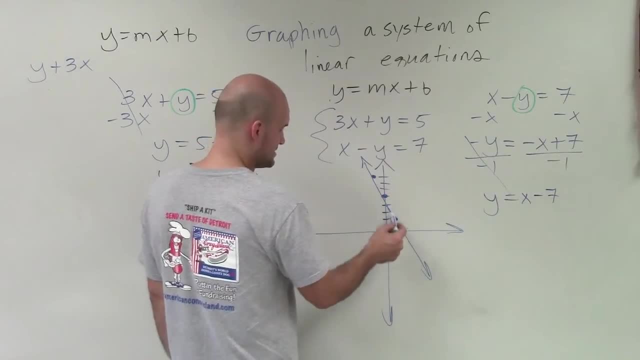 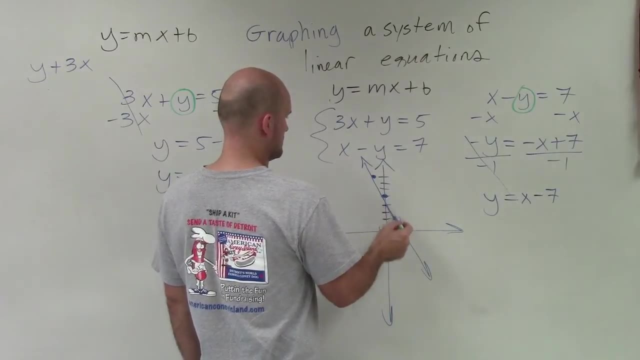 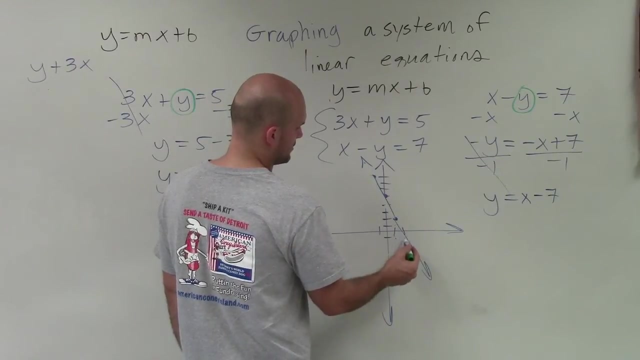 So Looks like I'm actually going to have to continue this. I'm down, so one, two. okay, I wrote this line really bad, Okay, so it's down. one, two, three over one. Down one, two, three over one. 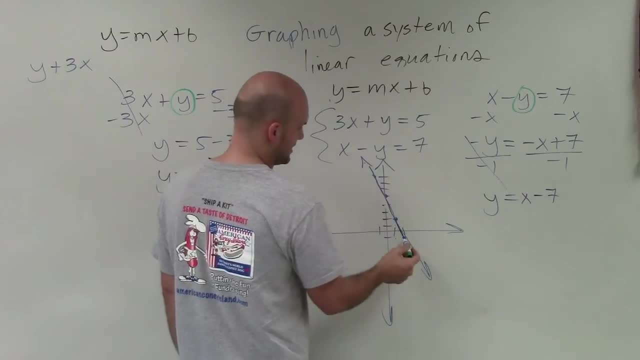 I'm just trying to get a good idea of what this line is going to look like, because I know I'm going to come down to it. That's down one, all right, so then down one, two, three to the right, one more. 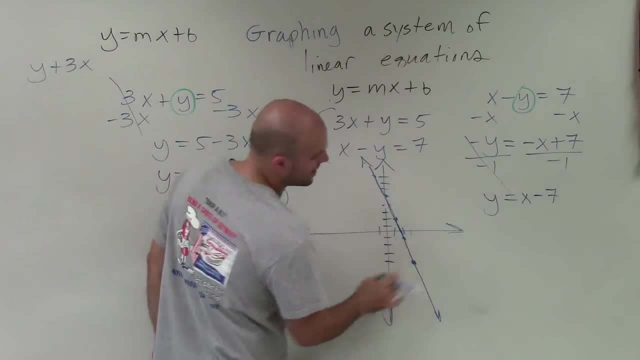 Okay, so just trying to get a better idea. That's why grid paper is really helpful. So now I go and graph this, which is down: negative seven, one, two, three, four, five, six, seven, And negative seven tells you to go up one right one up one up one right one up one right one. 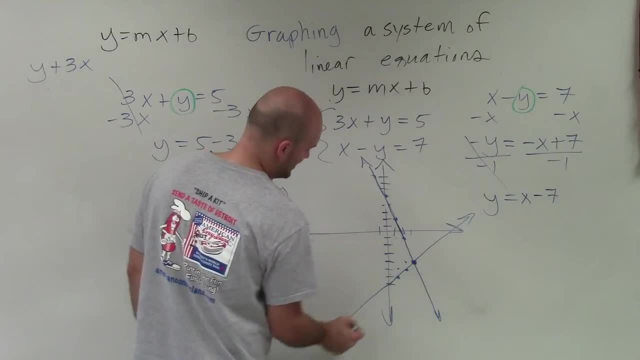 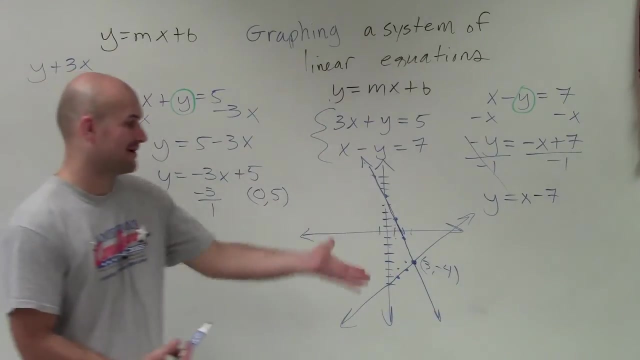 So I'm assuming, if I did my graph correctly, that I would have. now this point is going to be at this coordinate point which is over one, two, three, down one, two, three, four. So the intersection point, as long as I did my graphing correctly, is at the coordinate point three, comma negative four.